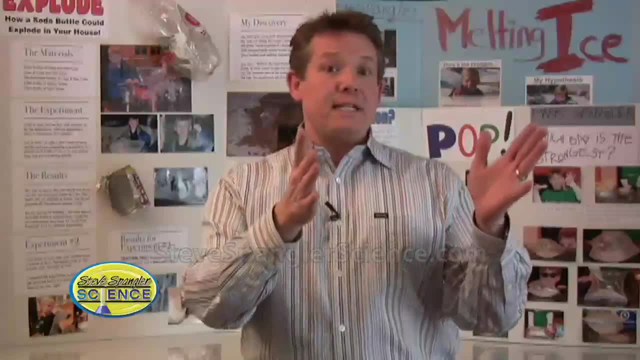 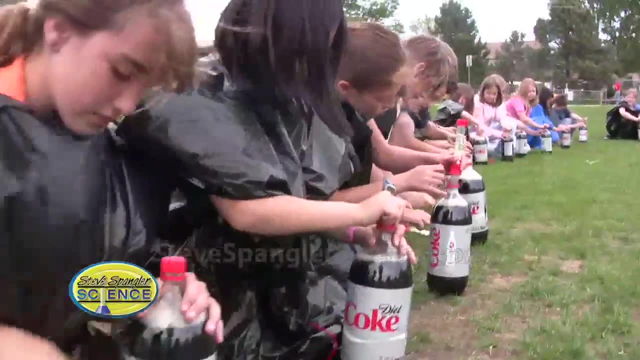 easy and I'll show you what you're going to do. You need to understand the difference between a science experiment, kind of a cool little activity, and an actual science fair project. You know, dropping the Mentos into the coke and causing the big eruption, that's. 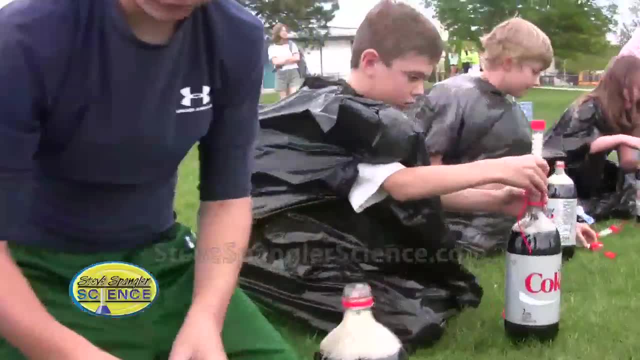 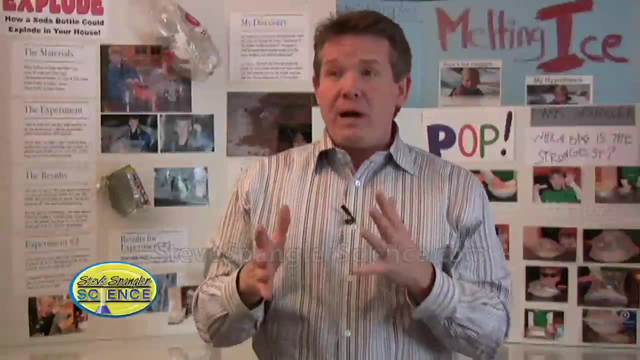 a pretty cool science trick, but if you want to turn it into a science fair project, you're going to have to incorporate some of your own elements: To count, compare, classify, observe and measure. You're probably going to want to set up some sort of comparison. So we all know that if you drop Mentos into soda, it's 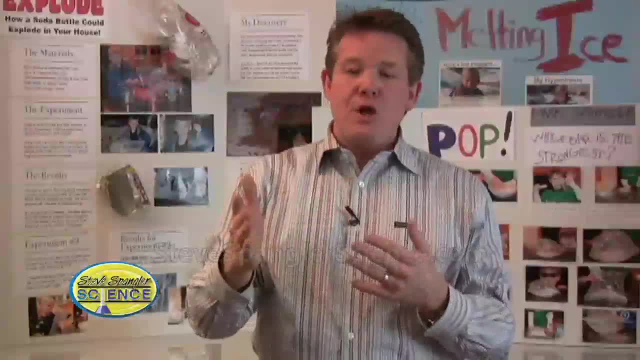 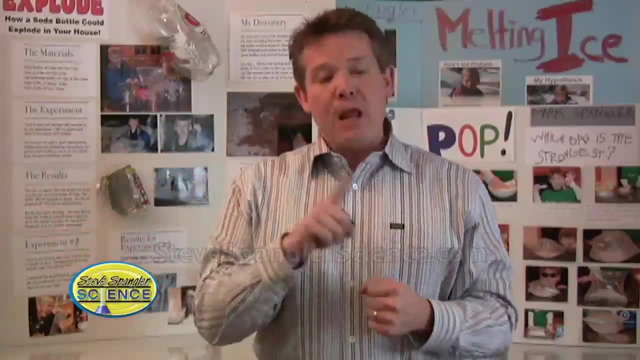 going to explode. but you have to stop and ask yourself some questions. What do you really want to know about that? How do we turn it into an experiment? that's actually a project that allows us to be able to compare some things. For example, you might want to know if I drop one Mento into a bottle of soda, will the geyser? 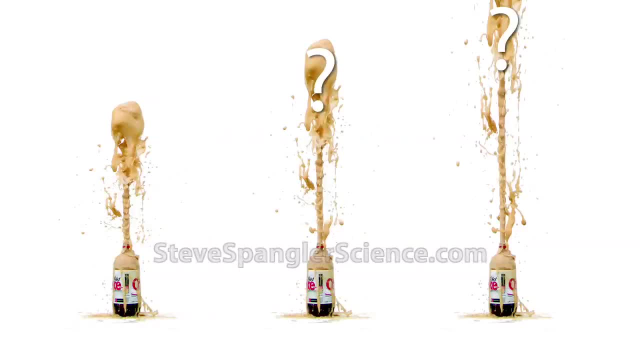 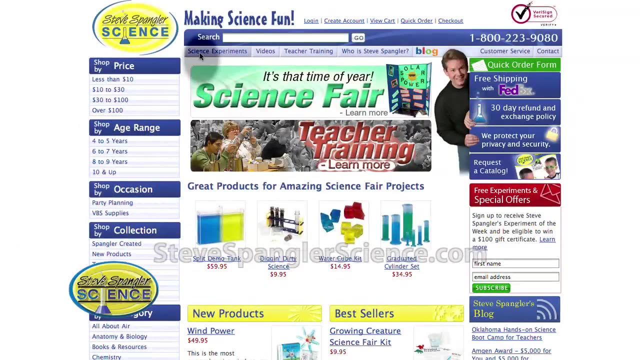 go up just as high as if I drop five Mentos. How about ten Mentos? You can see the comparison, but the important thing that you have to understand is that you can only change one variable at a time. So if you're going to change the number of Mentos, the type of soda. 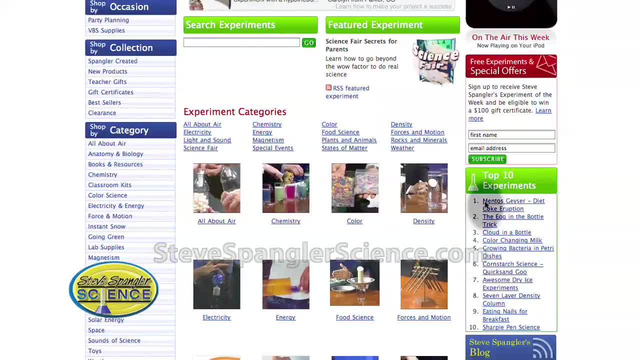 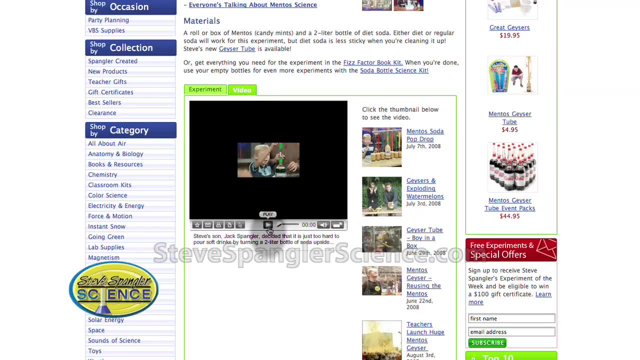 the temperature of the soda. everything has to stay the same. You have to just change one variable at a time to be able to do this for a science fair project. and it kind of makes sense as you look at all of the videos that are here and the experiment ideas that. 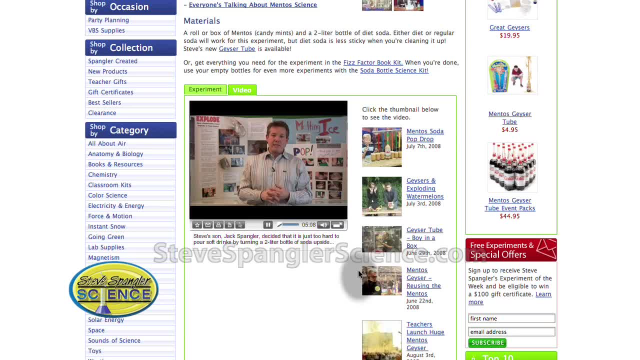 are here. You yourself have to make some of those changes and you're going to have a great science fair project. If you're a parent visiting our site, you're going to find some links below about tips for parents- Kids. if you're looking at the site and you're trying to come up with an idea, you might have. 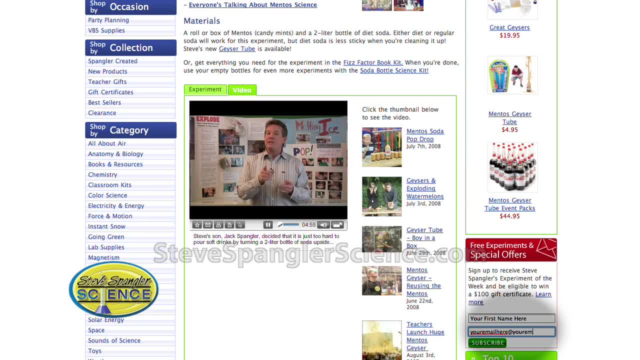 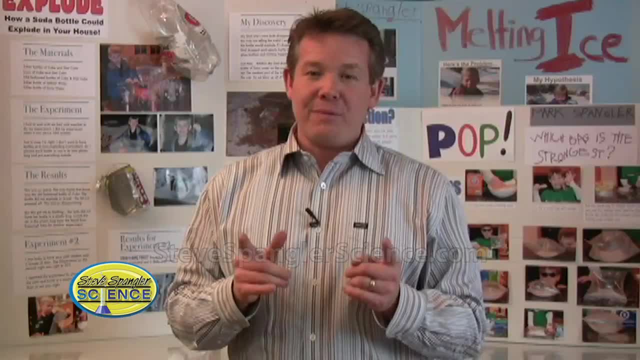 some ideas about formatting your science fair board that you see below, and if you're a teacher, there's some great tips here: how you can encourage your students and get the most out of them as we try to teach the scientific method. Well, it's time for me to stop talking. time for you to start clicking. Take a look at. 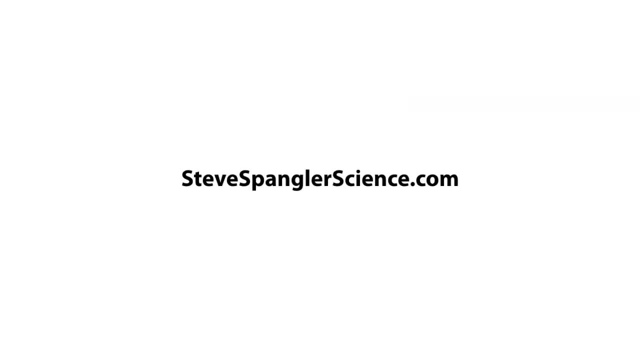 the videos, the experiments. you're going to come up with some great ideas. Have a great science fair.